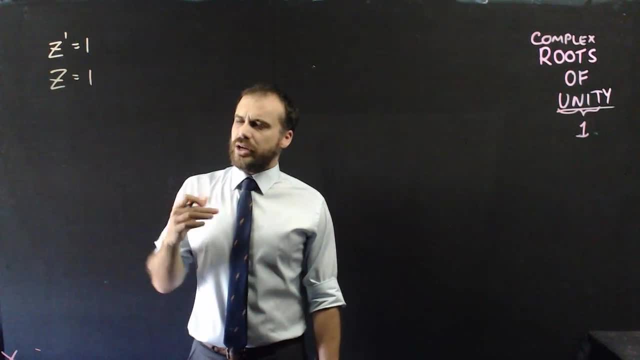 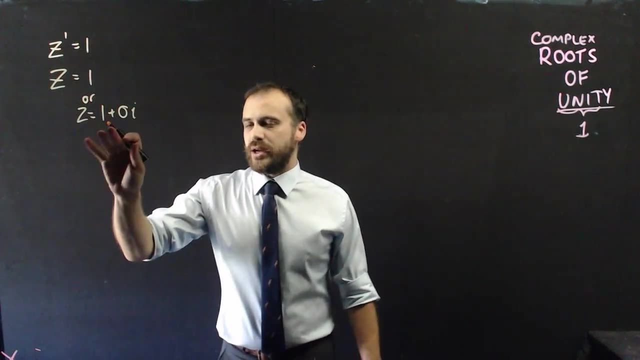 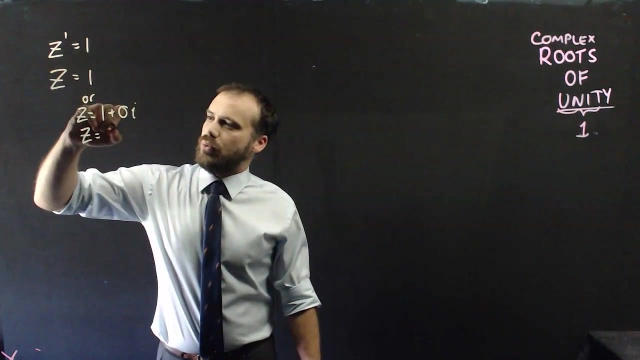 I could say that the answer is the number one. I could be more explicit and say that it's z equals one plus zero: One in the reals and zero in the imaginary. But I could also write that it's cis zero or one cis zero. 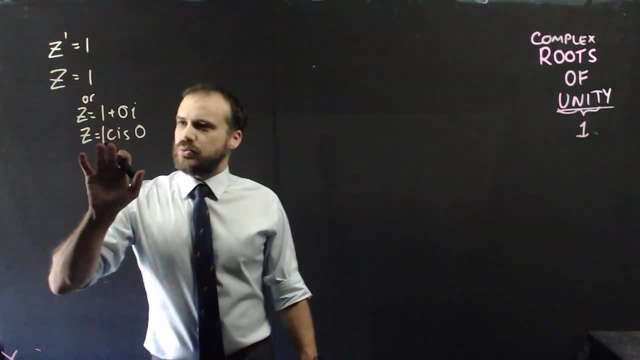 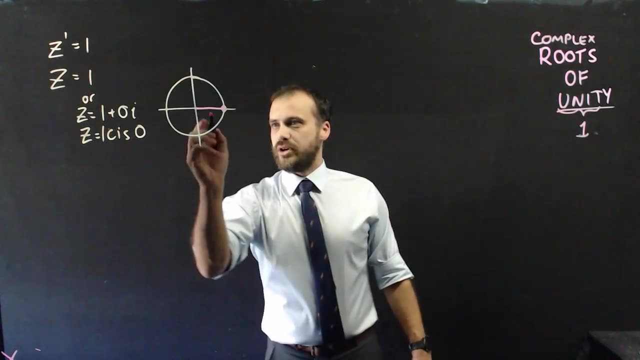 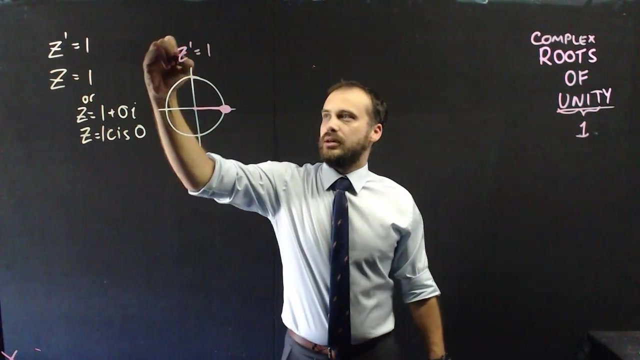 The one's not really necessary. That just says modulus one, angle zero, And I could draw this on an Argand diagram. So, Argand diagram, this is my one answer to the question z, to the one Equals one. Okay, what about the next step up? 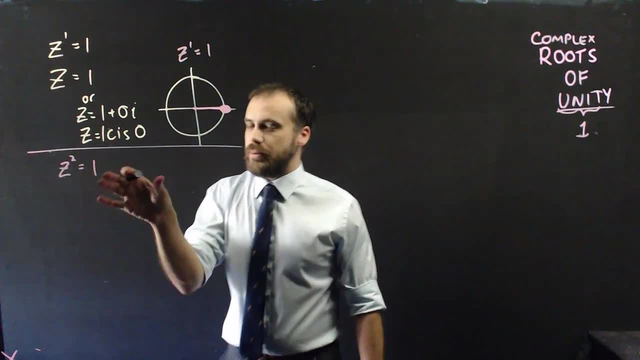 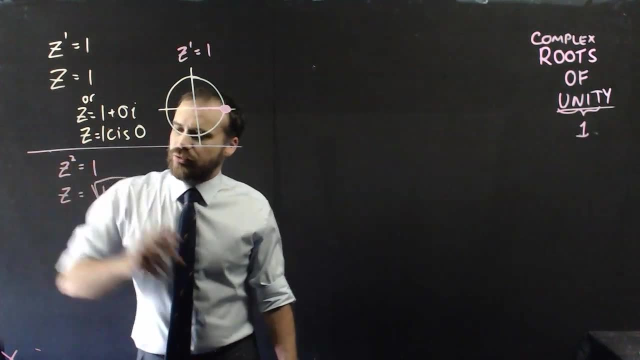 So we're doing another one here: z squared equals one. Now, remember, this is a complex number, even though it's purely real. So we're going to say that z is equal to the square root of one, But maybe we should think about it in a different way. 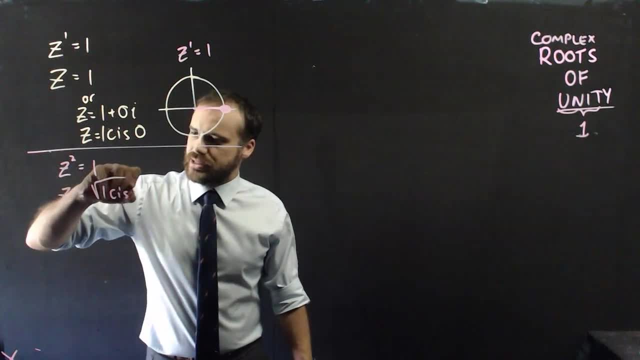 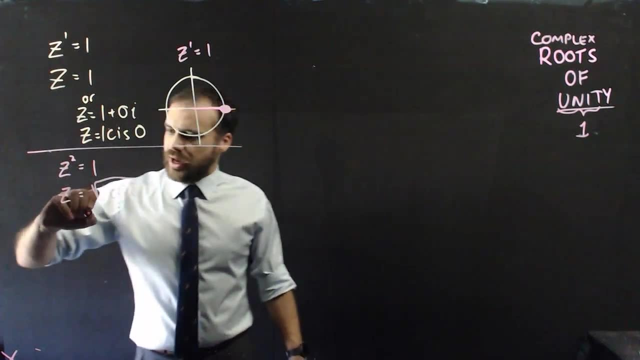 Maybe we should instead think about it as the square root of one cis zero, Because one and one cis zero are the same thing. We can then apply De Moivre's theorem here and say that that's the same as the square root of one cis. 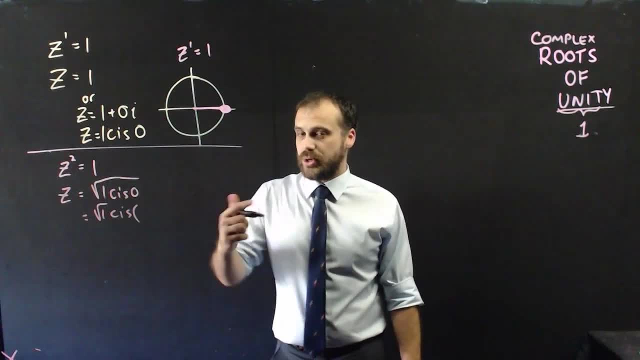 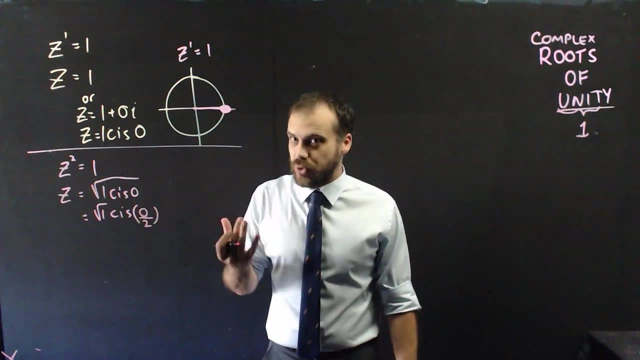 And how many answers are we going to get? We're going to get two answers, because we're taking a square root. Now, one of those answers is just going to be zero divided by two, which is, of course, zero. So that's one cis zero. 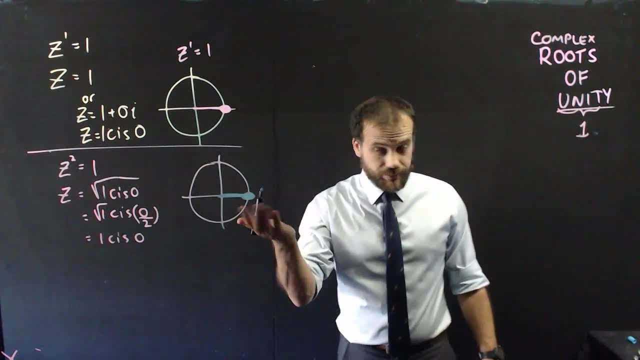 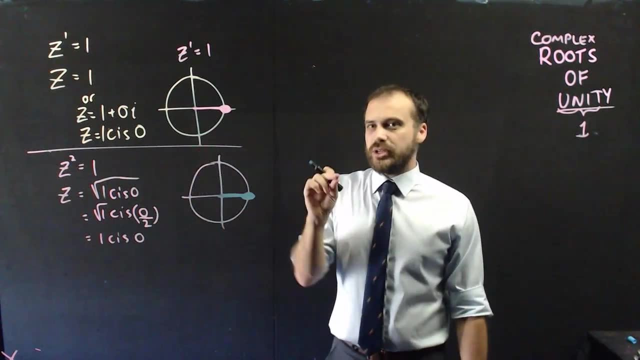 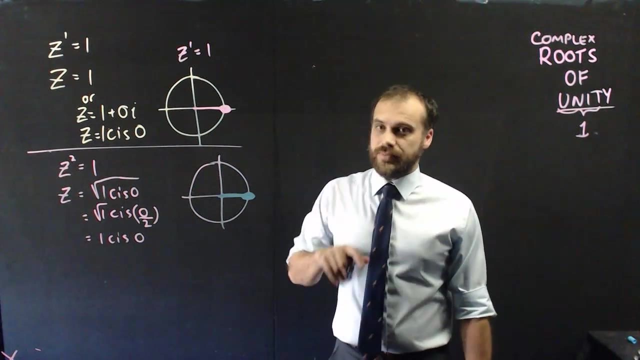 Which is, of course, one on an Argand diagram. Now, remember, when you take the nth root of a complex number- and one is our complex- you're going to get n evenly spaced answers on our Argand diagram. So that means I'm going to get two answers and they're going to be evenly spaced. 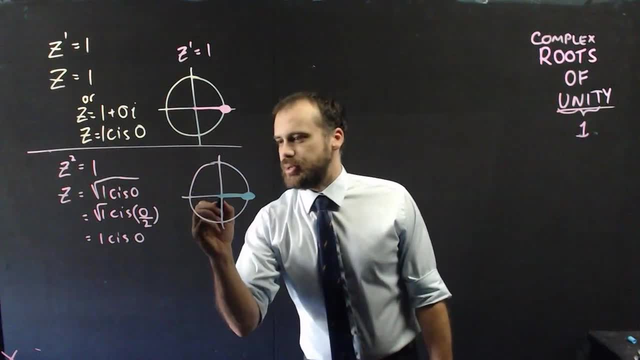 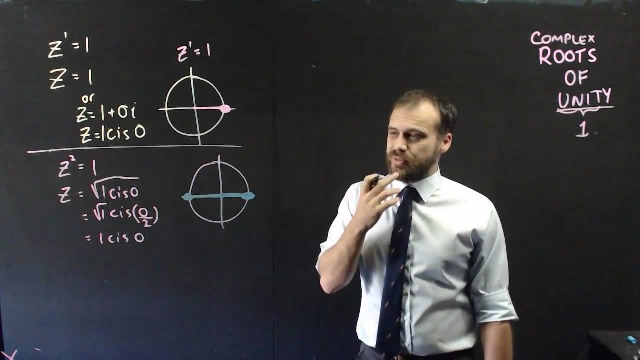 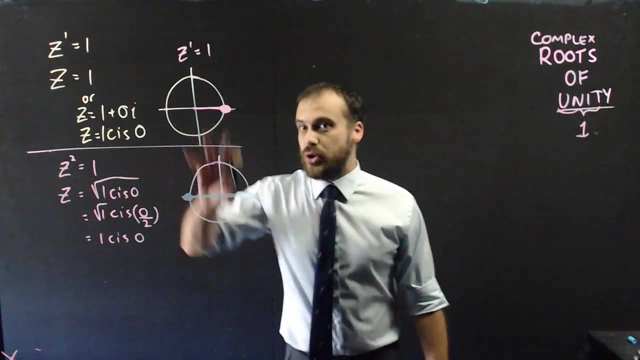 And one of them is there, which means the other one must be there. Okay, I have two answers now, and so far we kind of could have figured this out without complex numbers, Because our two answers are positive one and negative one. no imaginary components. 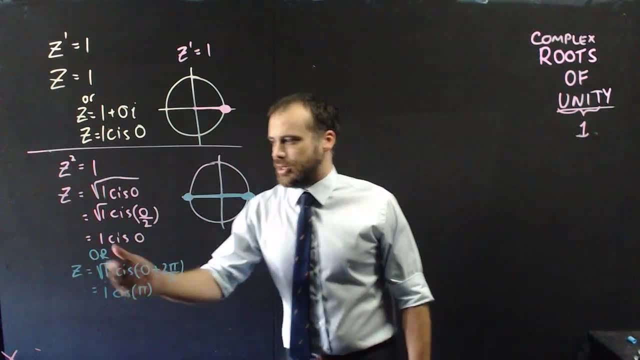 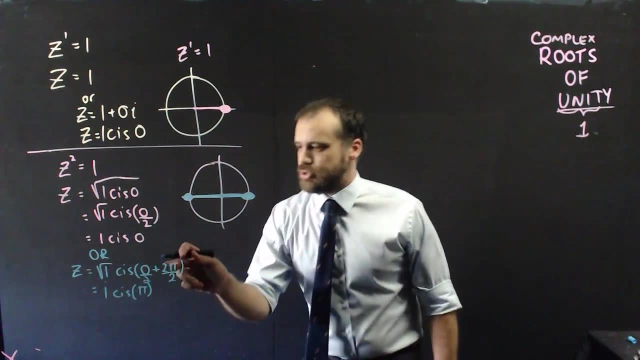 Just for the sake of thoroughness, I'll show you the algebraic bit here. So one of our answers was cis zero divided by two. The other answer is zero divided by two plus two, pi on two, which is one, cis pi, which is of course negative one. 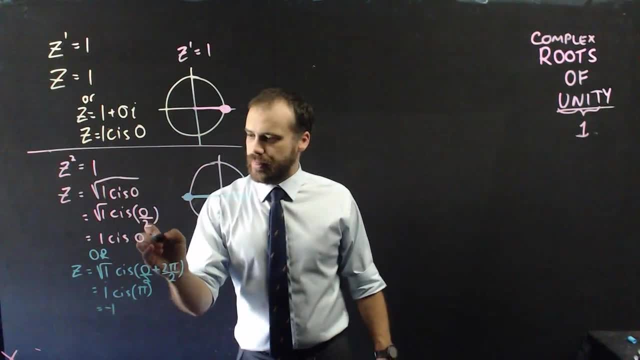 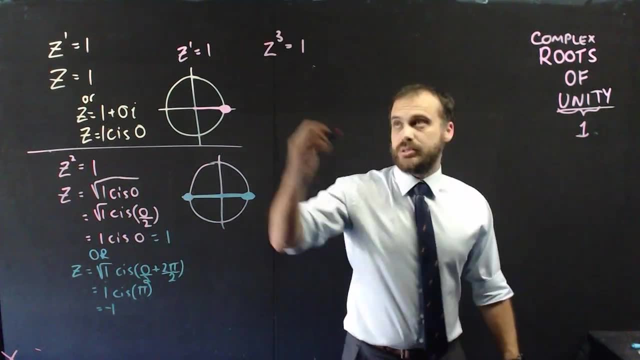 Which is our answer right here. So our two answers are the number one and the number negative one. Now z cubed is where it gets interesting. Now, z cubed is equal to one, so of course z is equal to the root of one, but let's treat it as a complex number. 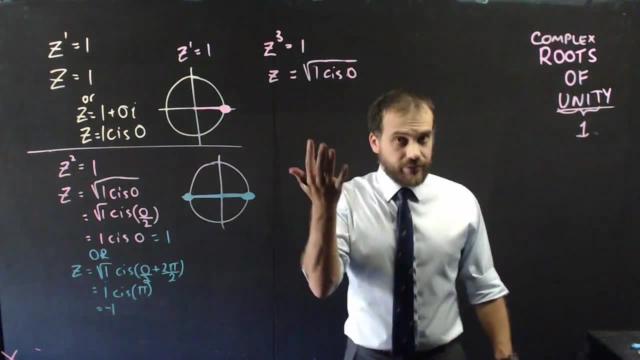 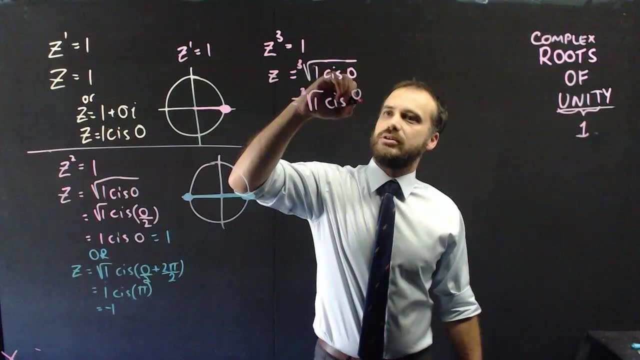 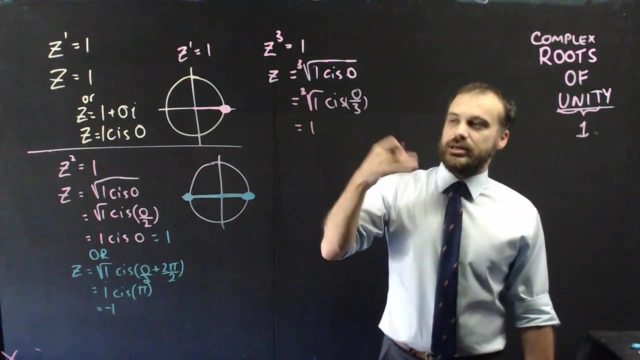 So one cis zero, zero. And we can of course use the Moivre's theorem here as well. Oh, that was a cube root, wasn't it? So cube root: one, cis zero divided by three. Now, of course, the cube root of one is one and cis zero divided by three is cis zero. 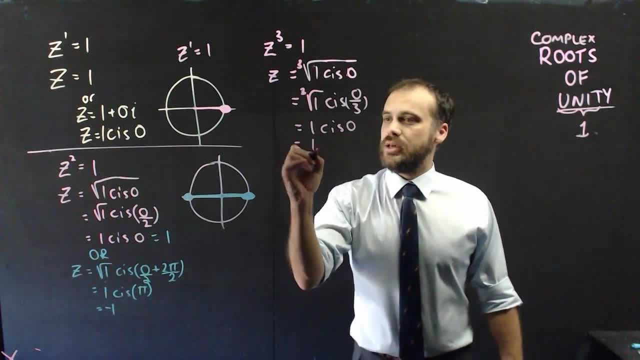 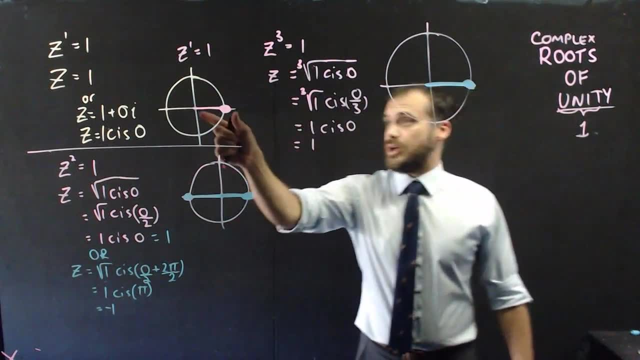 And by now we should know that one cis zero is just the number one, And on an Argand diagram we have that Now: z to the one, z to the two, z to the three. you can see all of our solutions. have one as an answer. 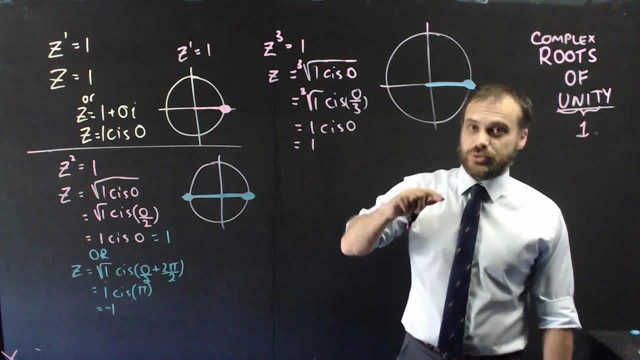 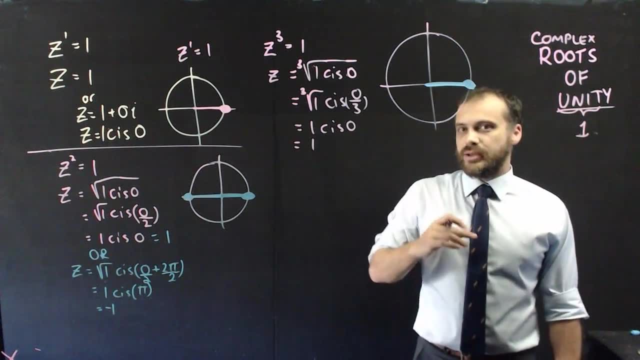 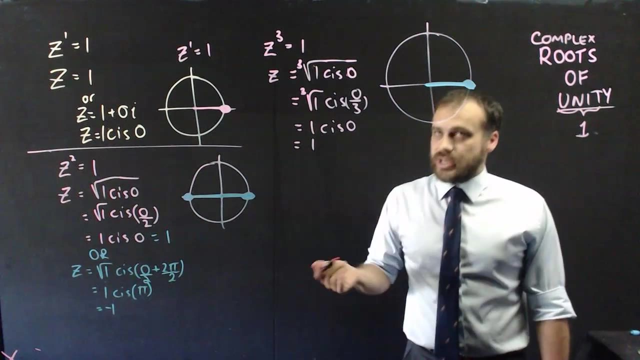 And that makes sense. Z to the anything equals one. One is going to be one of our answers. We always have an answer, a purely real answer: the number one. Now, we already know that when we take the nth root of a complex number, we're going to have n evenly spaced answers. 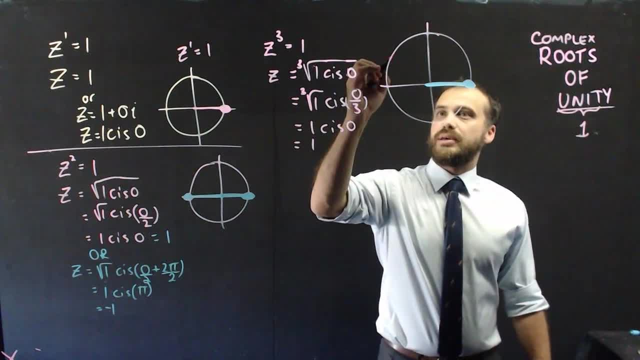 Which means that my other two answers are going to be here and here. So we're going to have n evenly spaced answers, which means that my other two answers are going to be here and here. I need to make sure that my angles are right. 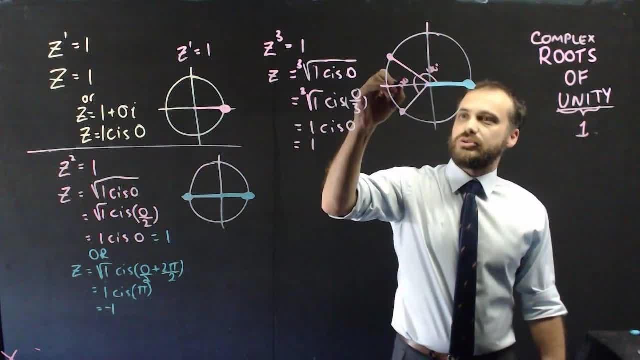 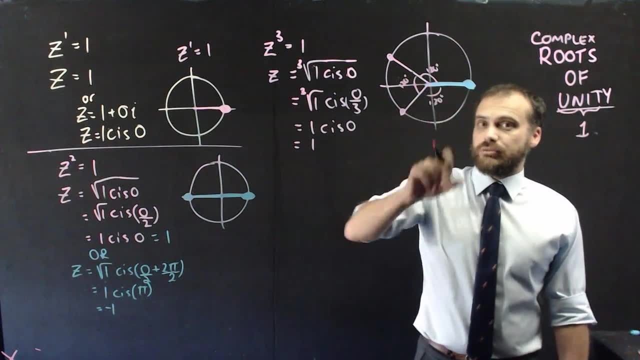 That's a 120 degree angle, and this is a 120 degree angle and this is a 120 degree angle. Three evenly spaced answers, one of them purely real one. Now, I've also given these answers in sort of purely algebraic terms here. 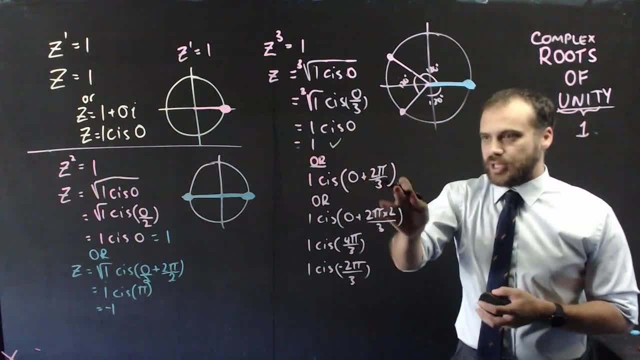 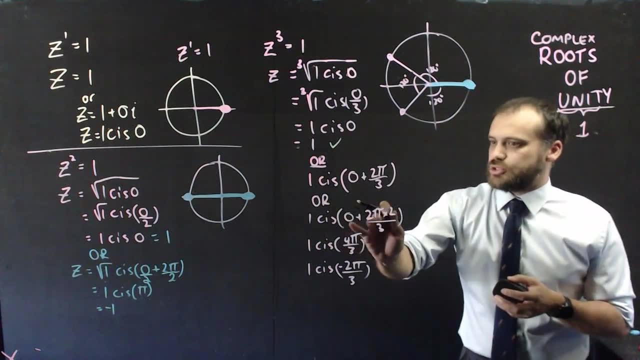 So one of the answers was one or one cis zero plus two pi on three, which is just cis two pi on three, 120 degrees. Or one cis zero plus two pi times two over three, which is cis four pi on three.